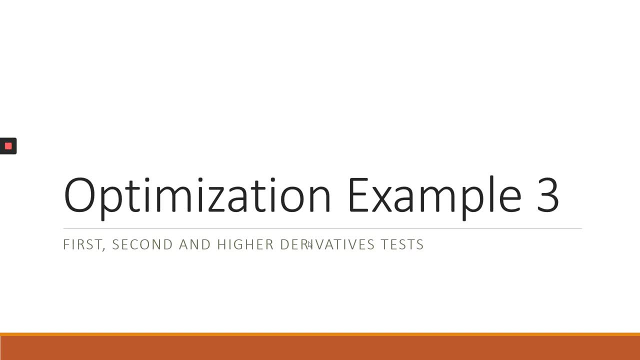 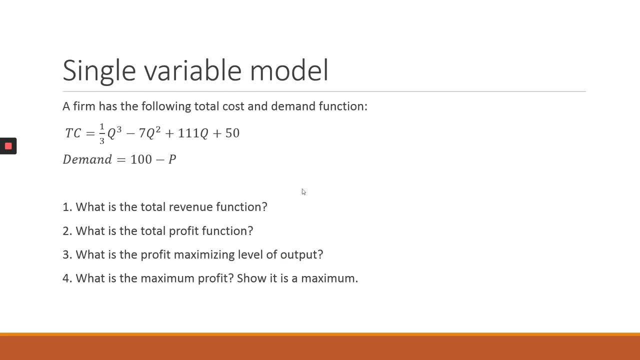 Example of optimization problem. In this example we are still working with a single variable model. So the problem says FM has the following total cost and demand function. Right, First question is: what is the total revenue function? The second question is: what is the total profit function? 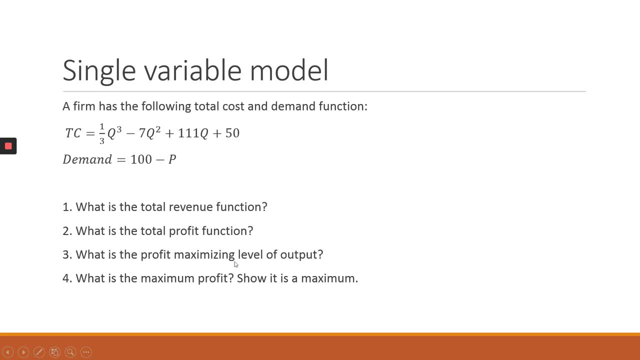 The third question is: what is the profit maximizing level of output? And the fourth question is: what is the maximum profit? Sure, it is a maximum, All right. So from the given information, basically we know that when we are calculating total revenue, we have to multiply quantity times price. 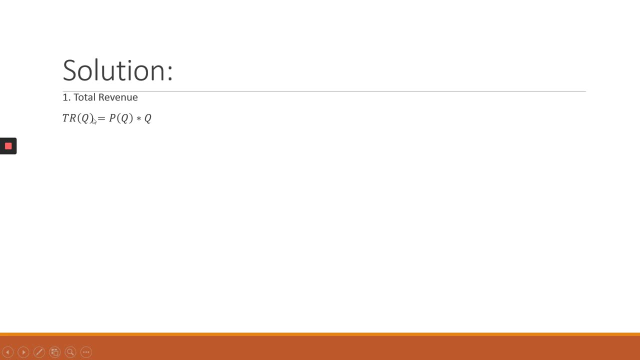 Right? So from the demand function itself. basically, it's defining Q as a function of P, But what we want in our total revenue function is to define a function in terms of Q, Right? So we need to get the inverse demand function and multiply it to Q. 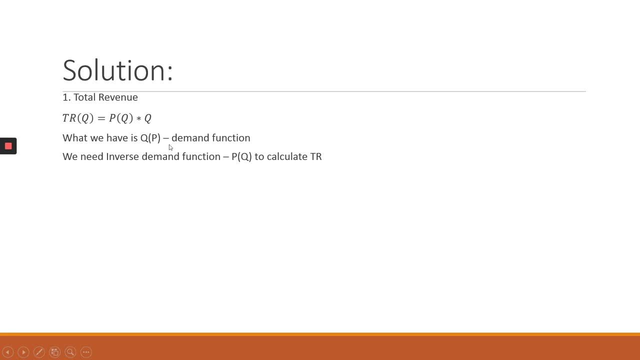 Right. So to get the inverse demand function. basically, what we're going to do is to rewrite the demand function Right, Right, Making P subject of the formula Right. So now we have P equals to 100 minus Q. So with the price now we can multiply it to Q to get total revenue. 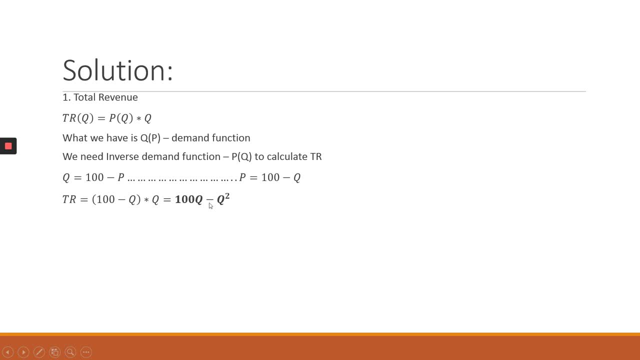 Right. So our total revenue becomes 100 Q minus Q squared To get the profit function we are going to use now, the new total revenue function we have derived together with the given total cost function. So profits is the difference between the two: total revenue minus the total costs. 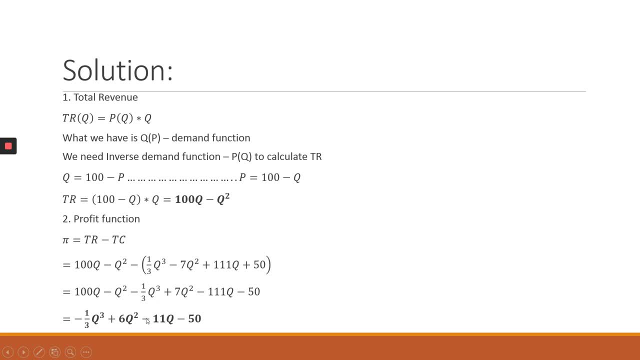 Right. If you open the bracket and simplify, we'll find our total profits. basically is equals to one minus one third, Q cubed plus six, Q squared minus 11, Q minus 50.. Right To calculate now the profit maximizing level of output as we have established. we have to find the first order conditions and set them equal to zero. right of our profit function.